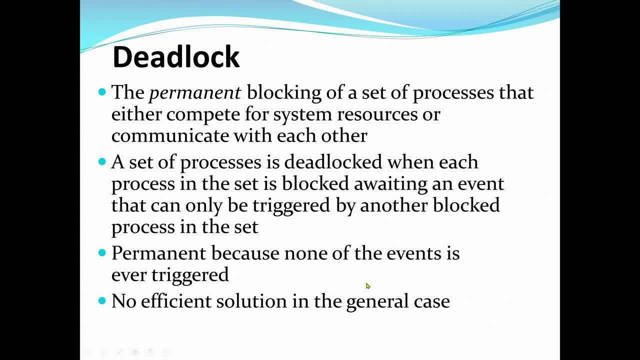 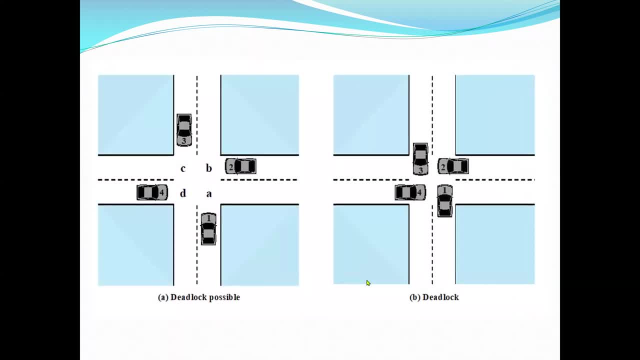 again, there's no efficient solution in the set general case. So here we have an example of a deadlock possible. We can see we have a four ways and as the cars are approaching the intersection you can see all of them want to approach at the. 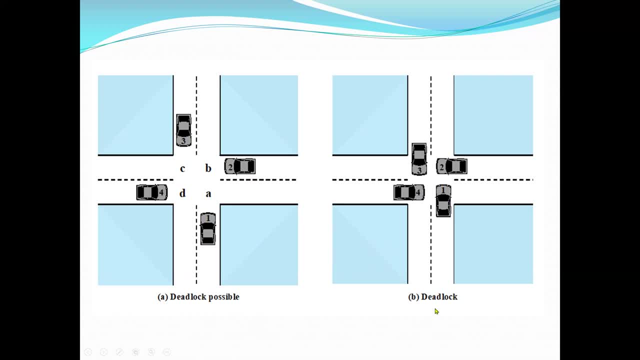 same time. And the second section. again we can see the deadlock. they all approach at the same time. So all deadlocks normally involve conflicting needs for resources by two or more processes. So when we have two or more processes and there's a conflict means for them, then there. 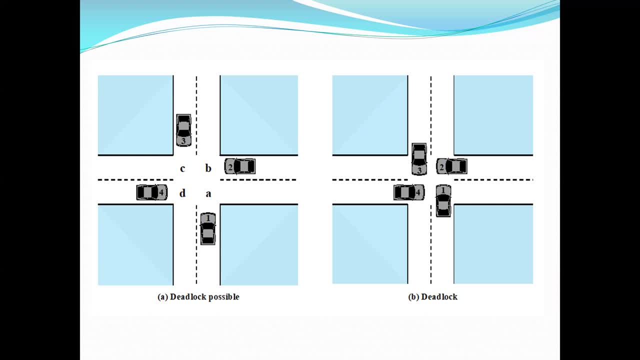 will be a deadlock Again. the common example, as we said, is the traffic deadlock, And the diagram shows a situation in which four cars have arrived at four-way stop intersection at approximately the same time. Now, the four quadrants of the intersection are the resources. 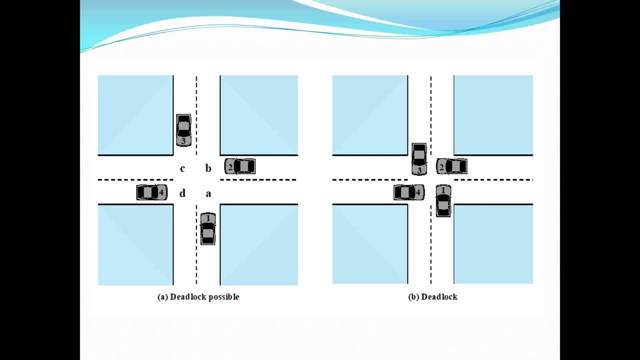 over which control is needed, In particular if all the four cars wish to go straight through the intersection. the resource requirements are as following. So let's say car one travel north in this quadrant A and B, And also car two needs quadrants B and C- Okay, B and C. And also car three will need a quadrant C and D. 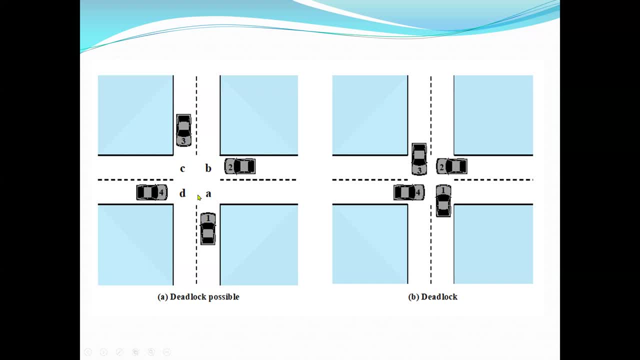 C and D. Then car four needs the quadrants D and A because it's going straight. So car one need A and B And four need D and A, Three need C and D And two need C and B. So the rule of the rules normally is that a car at a four-way stop should defer to a car immediately. 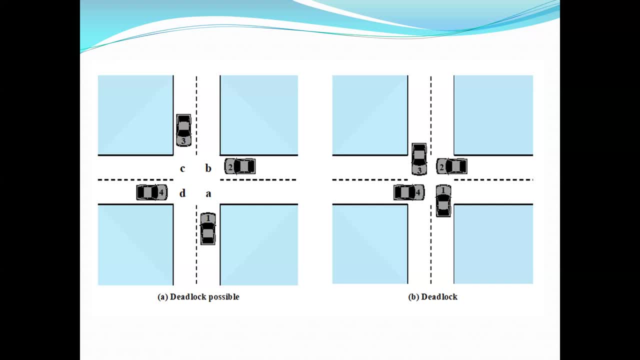 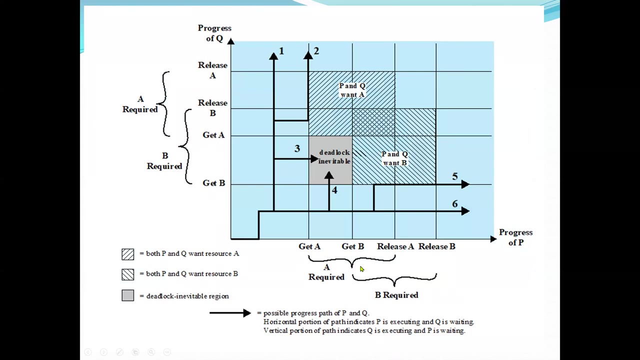 to its right, And this rule works if there are only two or three cars at the intersection. So again, that's the whole concept of deadlock. So, in terms of, again, resources, two processes: One to receive, or we want to keep the resource, and other processes, So the same resource you want to. 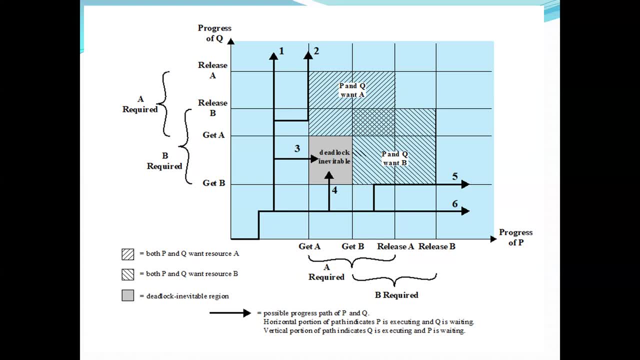 receive. So we have two processes. we want to use the same resource at the same time. If there's no communication can be a deadlock. so let's see this example. maybe we'll give a small detail now. let's look. look at this example here. so here we have something called a joint progress diagram. 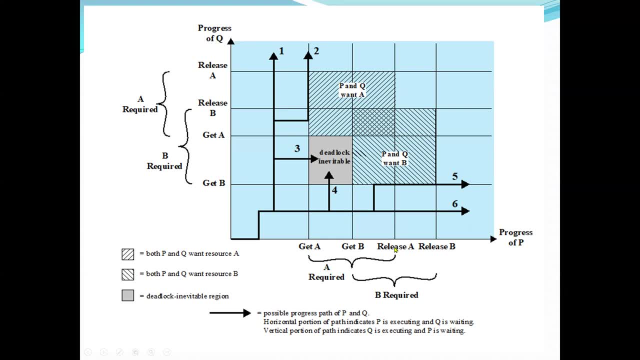 so we can see the progress of q, uh going towards our power. then we have the pro progress of p and to the lower right side. so we have a p and q at this section. we can see that again p and q and needs a resource at the same time. 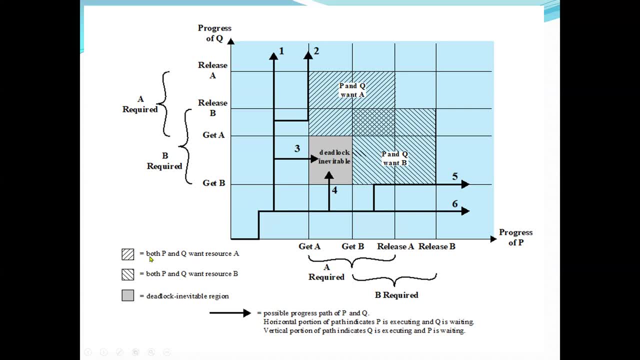 so the diagram show here. so both- the first dash of both p and q- want resources a. so p and q need resources at the same resources, a at the same time, and at this session also, p and q need resources b or 1b at the same time. 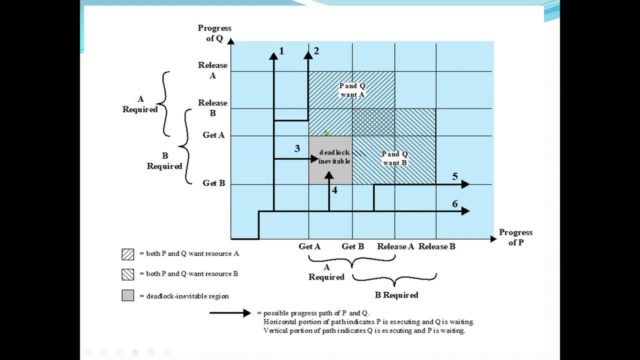 and here we're going to have a deadlock because we can see the two arrows coming towards. so here we say: the x, as is represent the progress at the execution of p- you can see the progress at the execution of p, as we said. and also the y, as is represent the. 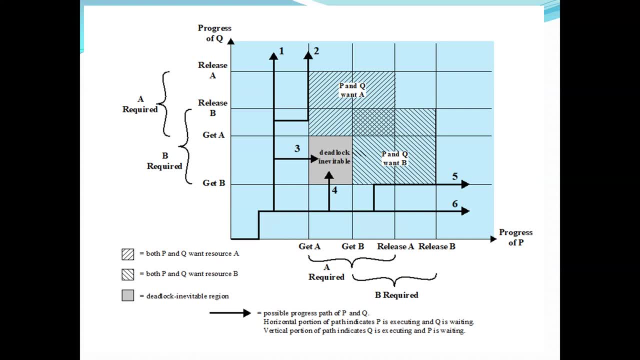 execution of q. now, the joint progress of the two process is therefore represented by a path that goes from the origin in the north eastern direction- so for uniprocessor system only one process at the time may execute- and also the path from the north eastern direction. 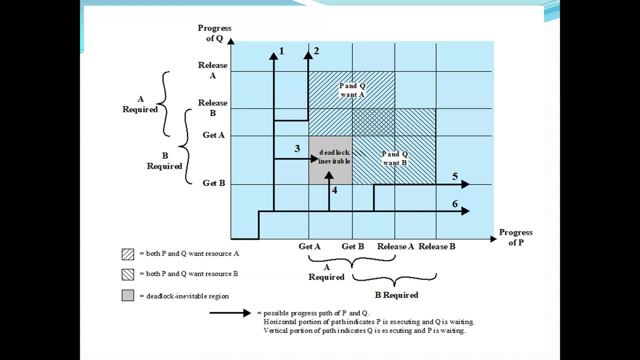 and the path consists of alternating horizontal and vertical segments, with horizontal segment represented representing a period when p execute and q waits, and the vertical segment will represent when q is acute. horizontal means when q azackit p weight. the figure indicates area in which both p and q require resources: a. so that's the section here. 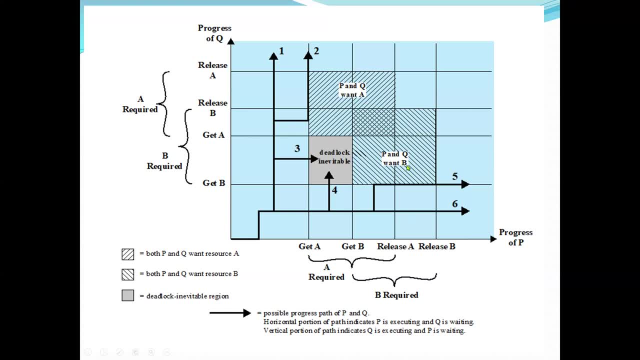 and also resources B of P and Q, Because we again assuming that each process requires excretion, control of any resources, these are all forbidden regions And that is, it is impossible for any path representing the joint execution progress of P and Q. 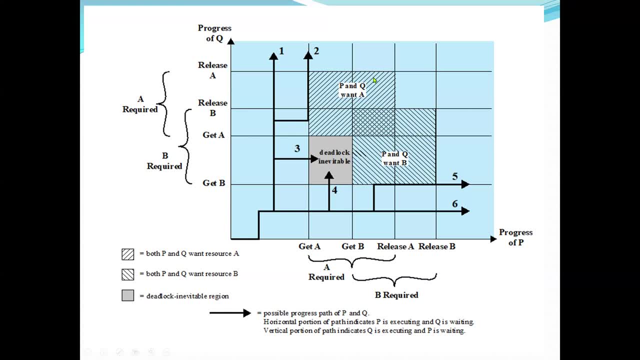 to enter this region. So the concept of, again, mutual excretion. So for example, here we can say that when Q acquire B, then A then release B and A, then when you release B and A, then one P will resume its execution. 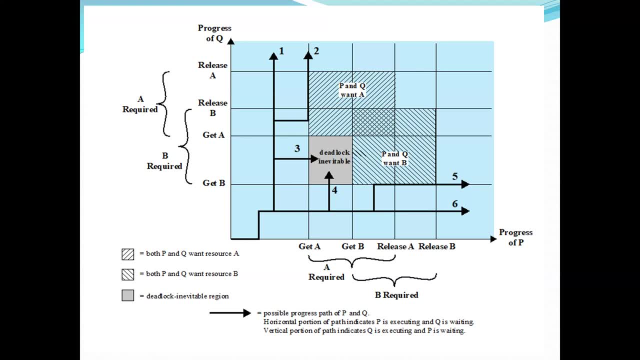 And it will be able to acquire both resources If Q again acquire B and then A and then release B and A when P resume execution, it will be able to acquire both resources because again, Q has released both of them. 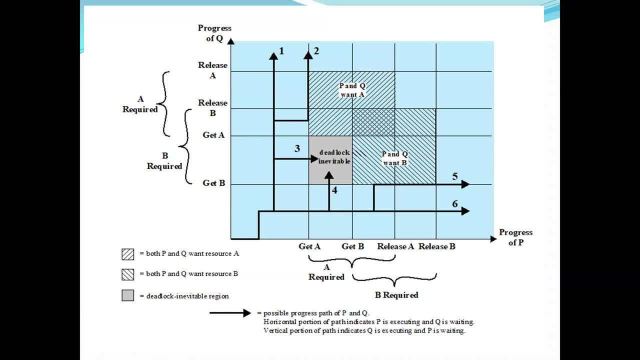 Now, when Q also acquired B and then A, P executes and blocks on the request for A. then Q releases B and A. when P resume execution It will be able to acquire both resources. That's, Q again acquires the B. 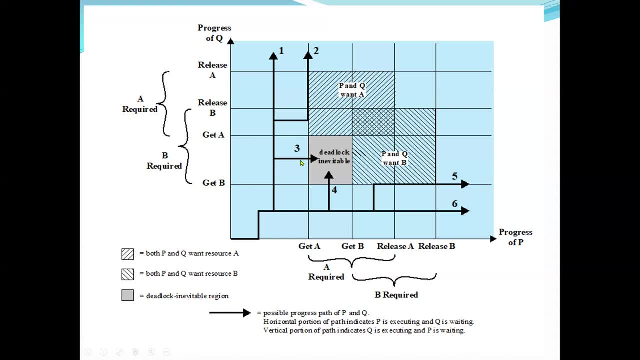 and then A, then P executes and blocks on the request for A. But when Q releases both B and A, then P can resume execution. So the whole concept we are trying to say here is avoiding the deadlock. If P is using the resources A, then Q have to wait. 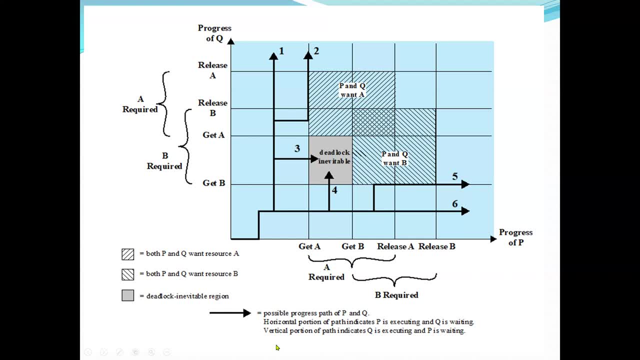 When P release it, then Q can use it. So in general we said here that if P is using the resources, they are waiting for A and they can still execute. They're waiting for A. So basically, if P is using the resources, 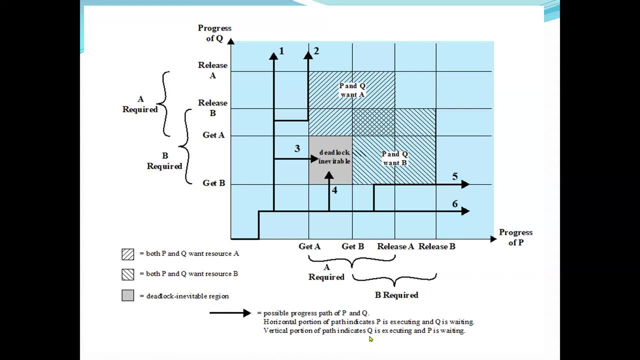 then Q have to wait for A until this point. Now the optimal head is the indication that P is executing, and if P is waiting for Q at the same time, then Q is executing. So when Q is executing, then Q is waiting for A. 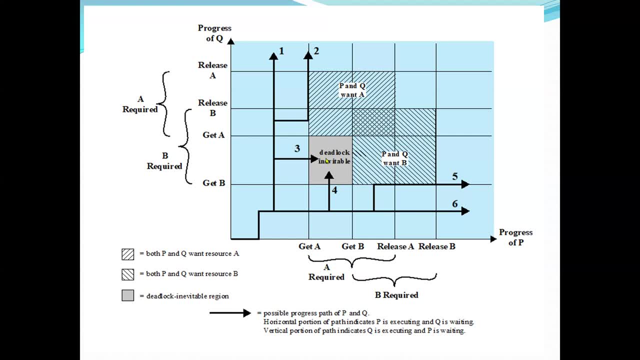 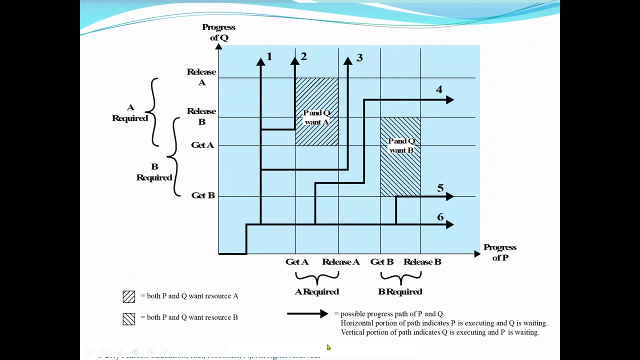 At least for the first five-to-six percent of the time. we will be able to see this when both, that's three and four- both of them may have deadlock or occur in this area. So, again, whether or not deadlocks occur depends on both, again, the dynamics of the execution. 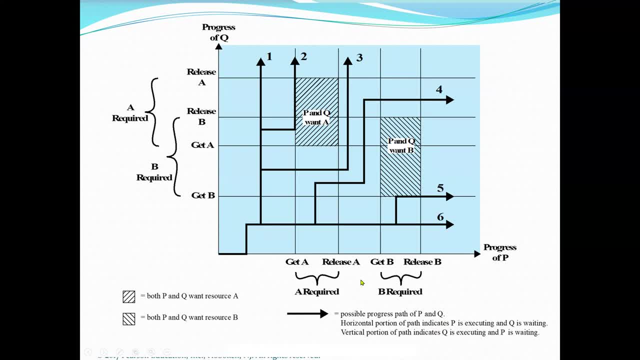 and on the details of the application. So again this situation is reflected, again this diagram. Some thoughts should be convinced as that, regardless of the relative timing of the two processes, deadlock cannot occur. So the joint progress diagram can be used to record the execution history of the two. 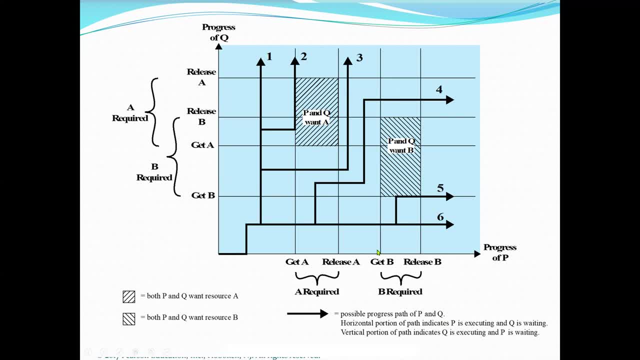 processes that share the resources. In cases where more than two processes are involved, deadlock is not possible. process may compete for same resource. then we need a higher dimensional diagram, required the principle of again concerning the fatal region, and that log will again remain the same. so here again we have both a and b want the resources a and both p and q want resources b. 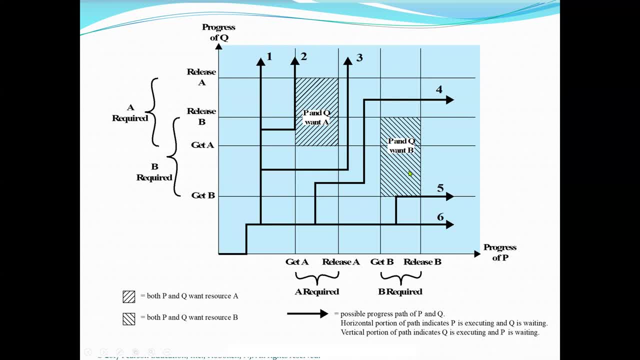 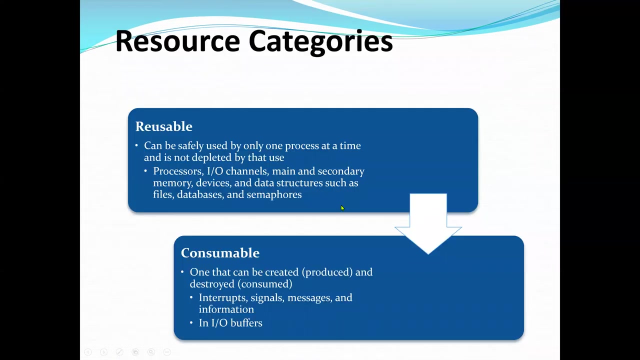 now in this area we can avoid a deadlock when p is executing again, as we said, q waits, key executing p with if they need that same resource. so here we can see: when b release, a will get it and keep going. so next we talk about the resources categories. 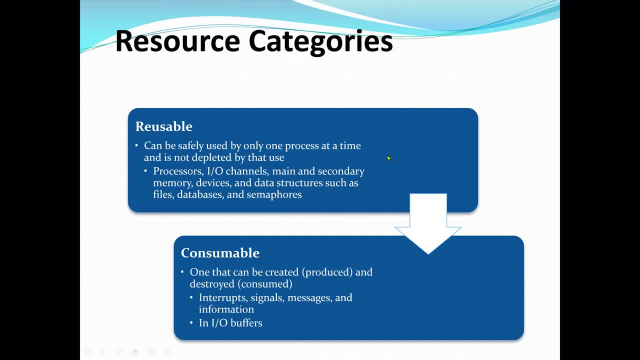 and here we say there are two general categories of resources that can be distinguished: we have the reusable and also we have the consumable. so a reusable resource is one that can be safely used by only one process at a time and it's not depleted by that use. 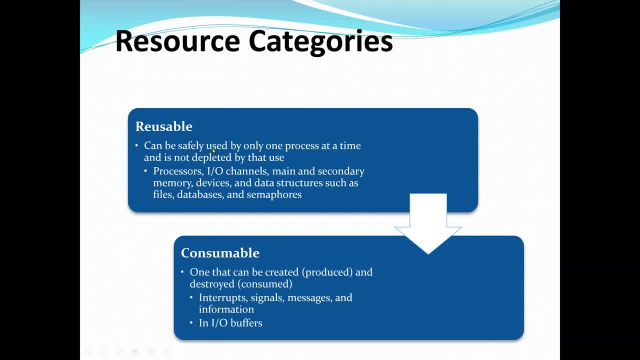 that's why, again, it's reusable, so this can be safely used by only one process at a time, and most of the processes that can be used by only one process at a time are not depleted by that use. now, processes obtain resources, units. that later relates for reuse by other. 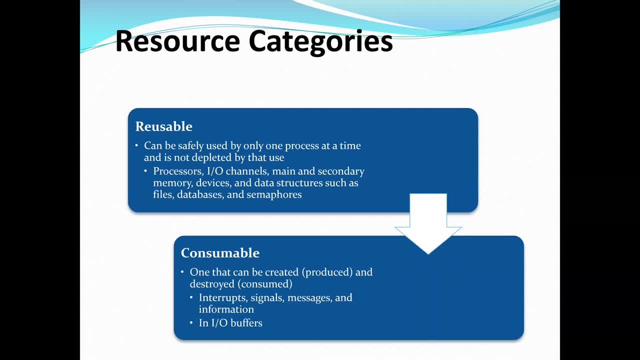 process. so example of reusable resources can include the processes or io channels, or even the main and secondary memory devices and other data structures such as file database, et cetera. Now, a consumable resource is one that can be created, that we can produce and also destroy, consume, 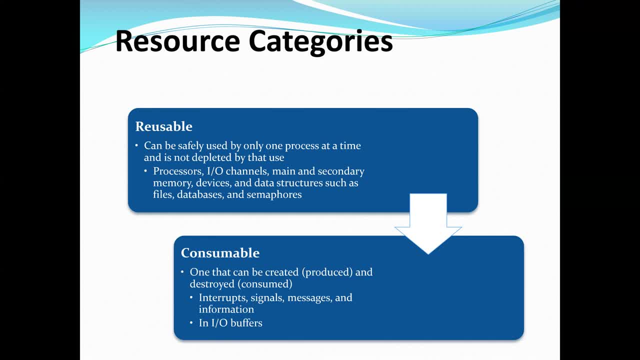 So example of a consumable resources are interrupts, sickness messages, informations and even the IO buffers. These can be created and also destroyed. So those are the two categories of resources. We have reusable resources, As we said. example can be the IO channels. 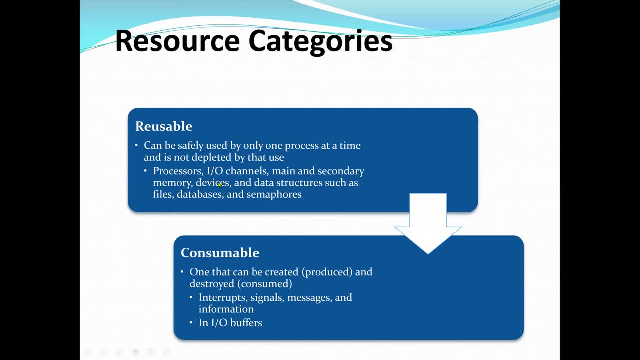 The main memory can be reused over and over Devices- example can be IO devices, the CPU, et cetera- But consumable again is the one that we can create and also we can destroy. So a very good example would be the interrupts. 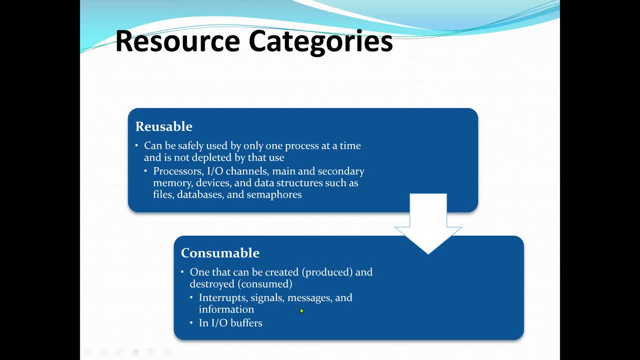 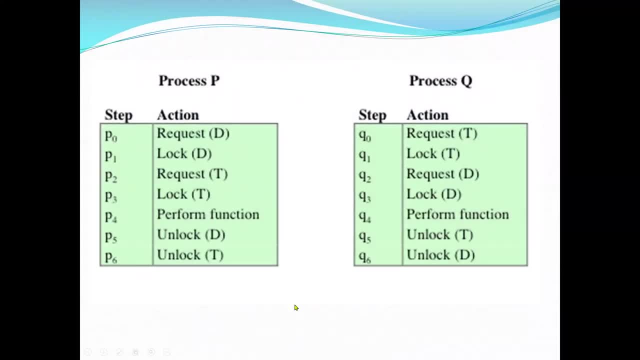 The sickness messages and informations. So we have an example here of a deadlock involving reusable resources. So consider two processes that compete for excessive assets to a DICS file, let's say file D. So we have the steps process PO up to P6.. 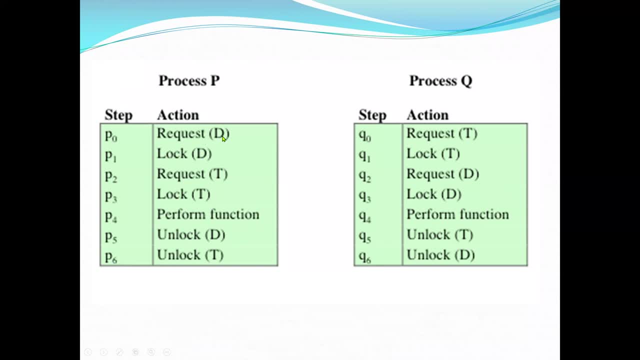 The action. first action is to request for the file D And also the tape drive T. So T represents our tape drive. So we have two processes: P&Q. so PO request first, Then when we request we lock it, then we request for T. 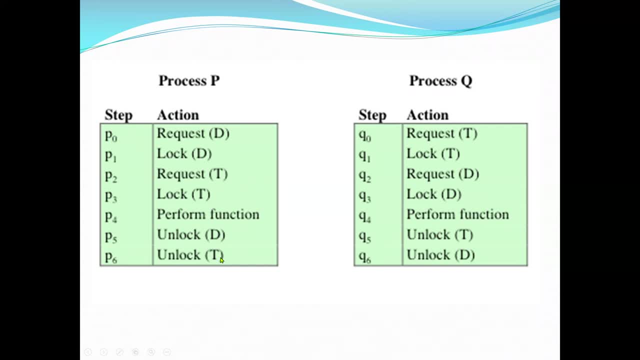 we lock it and perform a function and we unlock D&T. Now we then PQ field, PD, request T, then we lock T, then request D. we lock D, then perform action, then unlock T and then unlock D. So yeah, this is a very good example of involving reusable resources. 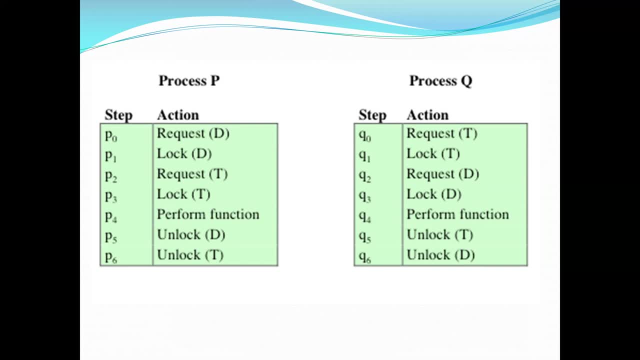 The program will engage in operation. that's shown in the slide here. Deadlock occurs if each process holds one resource and requests the other. For example, deadlock occurs if multi-program system interleave the execution of two processes as follows. So let's say: 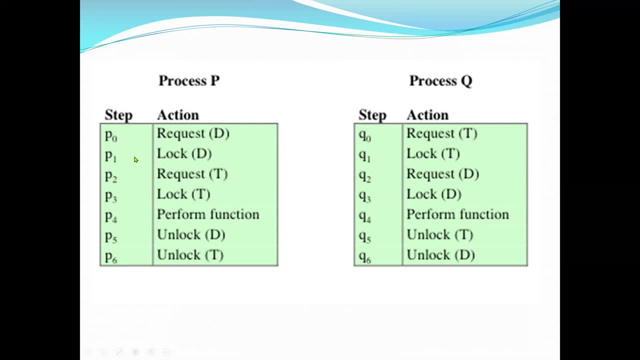 for example, we have P0,, then we have P1,, then Q0, Q1,, then P2, Q2.. Again, that will be a deadlock worker. So if I have these two, for example, process Q have requests for T. 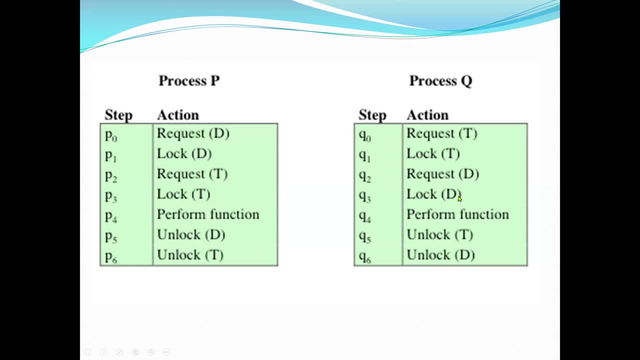 and you have T and it's requesting for D also, but it's not releasing the T. So this may appear that this is a programming error rather than program of OS designer. However, if we have seen that concurrent program design is challenging, then such deadlocks do occur and the cost is often embedded in. 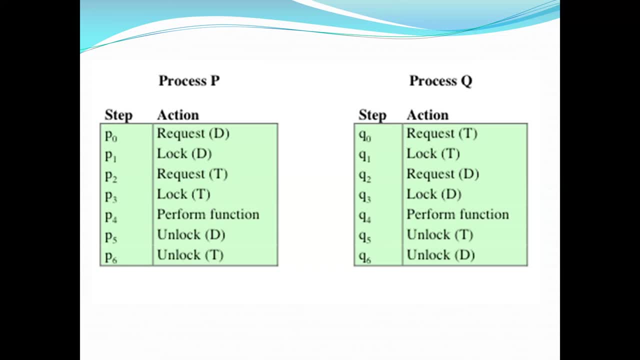 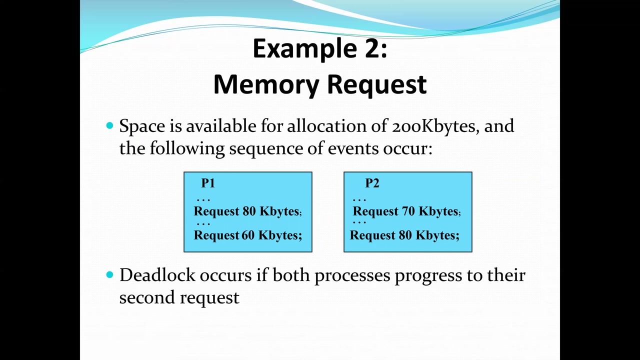 compressed program logic, again making detection difficult. One strategy for dealing with such a deadlock is to impose a system design constraints concerning the order in which the resources can be requested. I think that's very important to avoid a deadlock. Another example here of a deadlock with reusable resource has to do with the request for main. 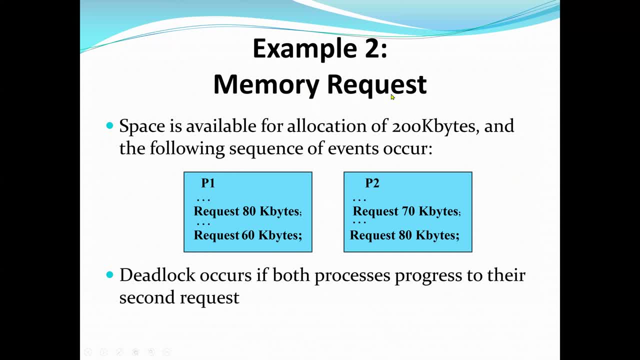 memory here. So memory requests. Suppose the space available for location is 200 kilobytes and the following sequence of requests occur: So we have P1, then request 80 kilobytes, request 60 kilobytes. 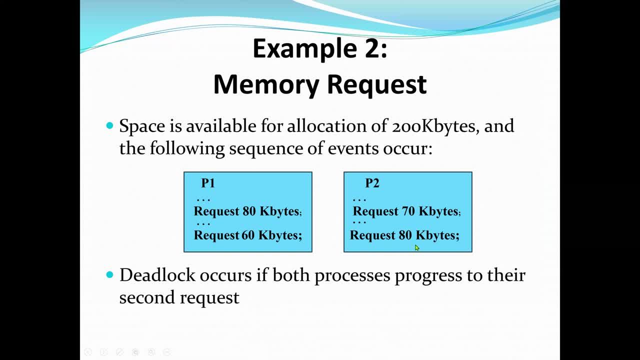 P2, request 70 kilobytes and request 80. 때도 Remember we have 200.. Now a deadlock occurred if both processes progressed in their second request, because here, if the amount of memory to the request is not known ahead of time, there is chance for deadlock to occur after the other processes completed. Again in today's presentation. here is the result of a deadlock and individual requests that unique for consuming time of memory. based on the rest of the gave data, the other requests have be Vorabis, Winji and Milorees. Quibastt allows the forward attributio. 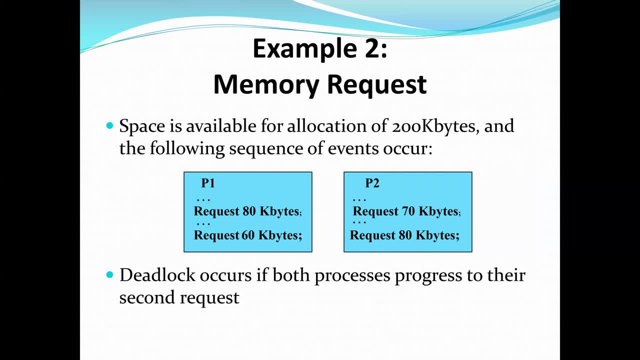 deadlock occurs if both data processes progress in their second request. Because if here, if the amount of memory to be requested is not, if the ability to access data is known ahead of time, request says it's not known ahead of time, it is, it is very difficult to deal with this type of deadlock. 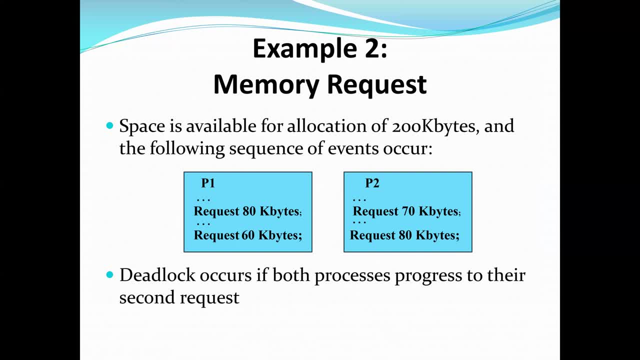 by means of system design constraints. so, again, the best way to deal with this particular problem is, in effect, to eliminate the possibility by using venture memory, which, again, we're going to discuss in our future lectures, and the problem here that we don't know the actual size from. 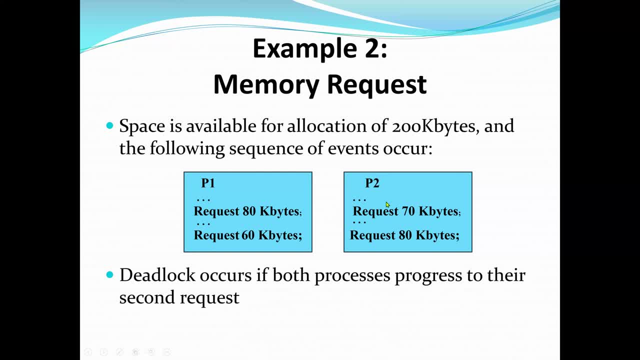 beginning. so we have 80, 70. the third time that's 150. the third time we are having 60 and 80. it passes the 200, the limit. so a deadlock occurs in both process, in both process. progress to the second request. now, if the second request is, let's say, only 10 kilobytes, 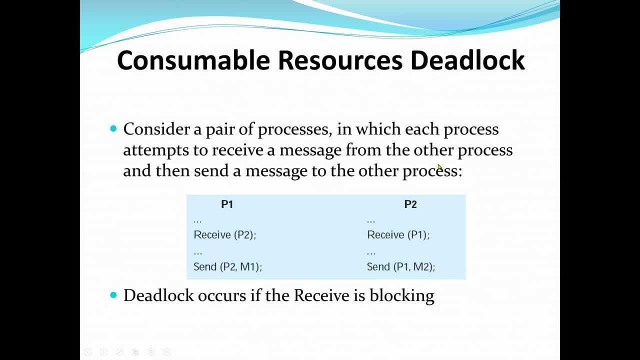 then it's within the 200 range, so that should work. now the consumer will resource deadlock. here we consider a pair of process in which each process attempt to receive a message from other process and then send a message to the other process. so we see the same. 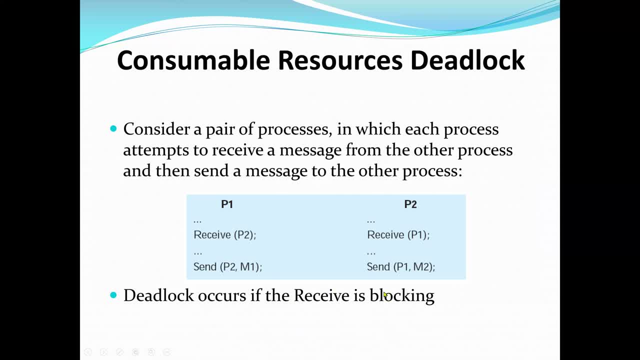 deadlock occurs if the receive is blocking. so this is again an example of a deadlock involving the consumable resources. that network again occurs if the receive is blocking. the receiving process is blocked until the message is received again. once again, a design error is the cause of the deadlock. such error may be quite difficult to 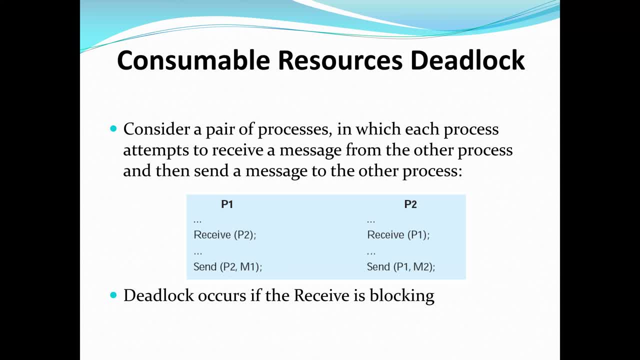 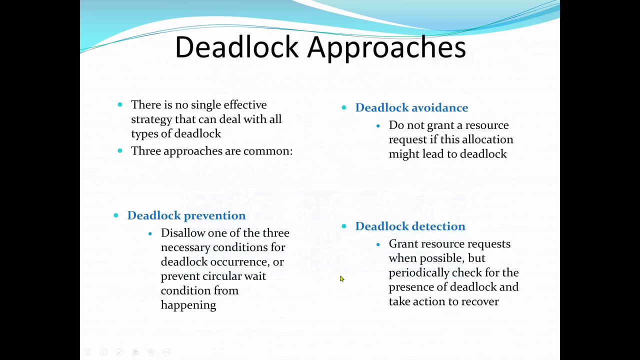 detect also. furthermore, it it may take a real combination of events to cause the thread, a deadlock. thus a program could be in use of a considerable period of time, even years before the deadlock actually occurs. so again, deadlock approaches. yeah, we say again, there is no single effective strategy. 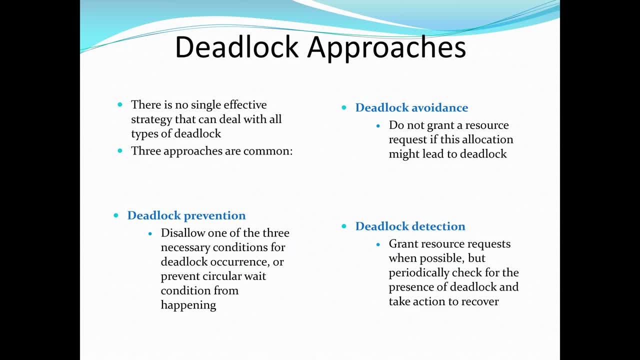 that can deal with all types of deadlock. we have different types, but we have three approaches that are very common here. the first is the deadlock prevention. this will disallow one of the three approaches- necessary conditions for deadlock occurrence or prevent circular wait condition from happening. And deadlock avoidance. here we make sure that we do not grant a resources request if 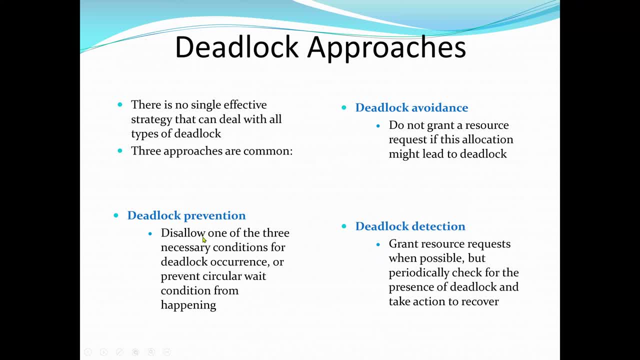 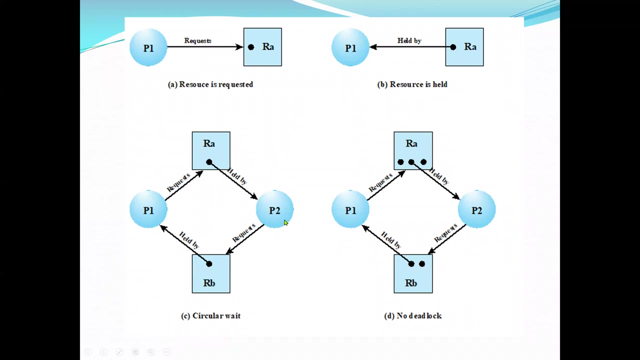 this allocation might lead to again deadlock. And then the deadlock detection. we should grant resources, requests when possible, But periodically we need to check for the presence of deadlock and take action to recover. And again, we are going to examine each of these in turn and in our few slides to come. 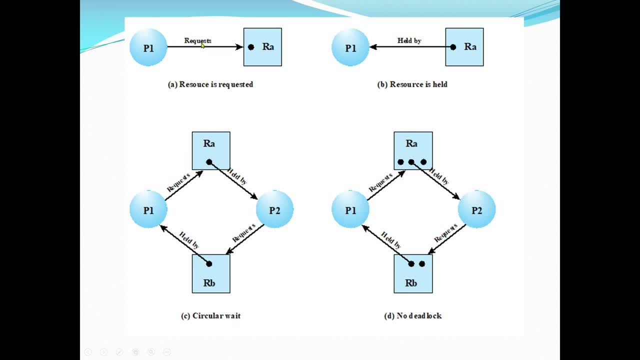 So here we can see A. we have P1.. We are requesting the resources RA, so resource requested And the resource is heard by P1.. Now in a circular wait we can see P1 requests for resources, but P2 is heard by it. 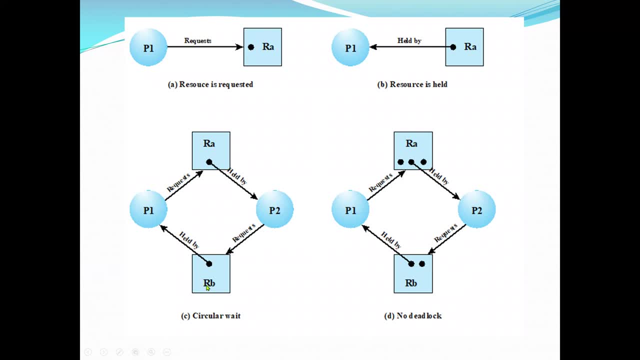 And also P2 requests resources of A Rb and also is heard by P1.. So process one needs some resources but is heard by process two. Process two also needs some resources, but that resource is also heard by process one. So this is called the concept of again circular wait. 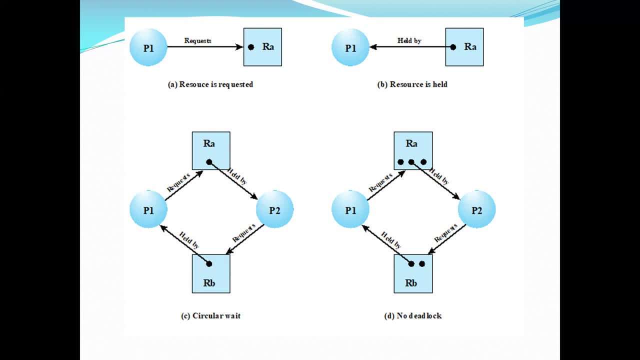 So again, the useful tool in characterizing the allocation of resources to process is the resources, the resource allocation graph. So the resource allocation graph is a directed graph that shows a state of the system of resources and process, with each process and each resource represent by a node. 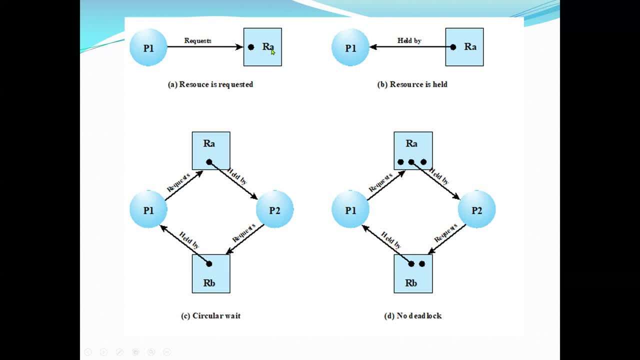 So here we have a node for P1 and RA. So the graph edge, directed from a process to resources, indicate the resources that has been requested by the process but not yet granted. So example will be A. this is a directed graph, is requesting but not yet granted. 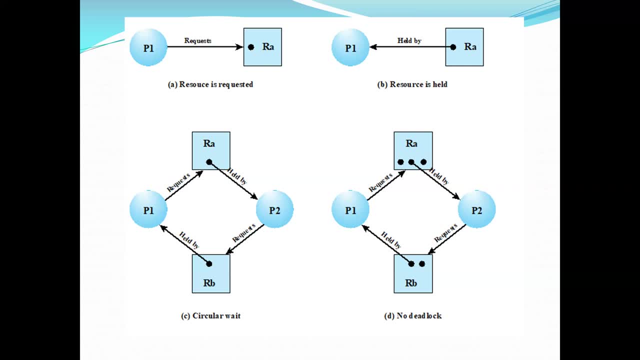 B within the resources node the dots show the instance of that resource. So in B the resources again is granted. The graph edge again directed from reusable resources, that's reusable resources. RA is directed towards the process. indicate that the resource has been granted. 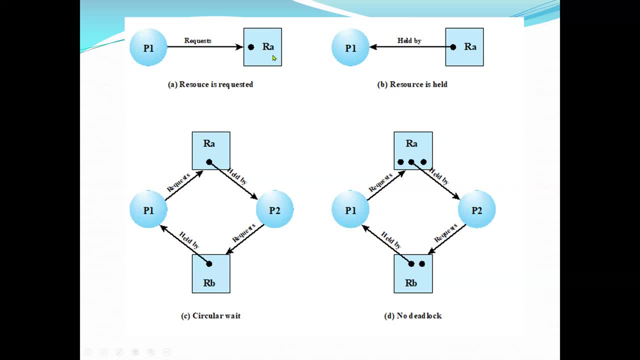 So again, we may see the examples of this in our future slides soon. So C: again it's got a circular width because circular width is the mode of the nodes. it's here we can see that there's only one unit each of resources, re and rb, but process one. 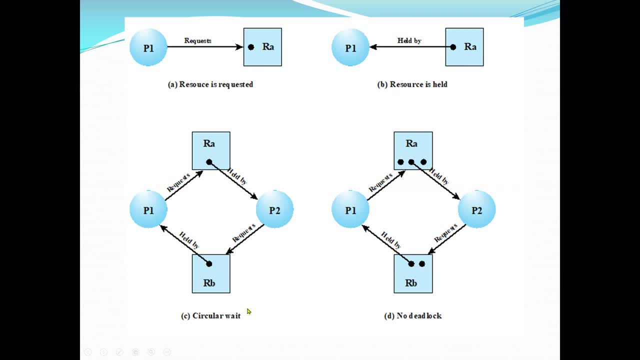 or i'll say: p1 owes the rb and requesting array yp to also hold r a by requesting for rb. so we have the idea of the circular weighting, but in this case there's no deadlock because multiple units of each resource still available, and that's the whole concept here. 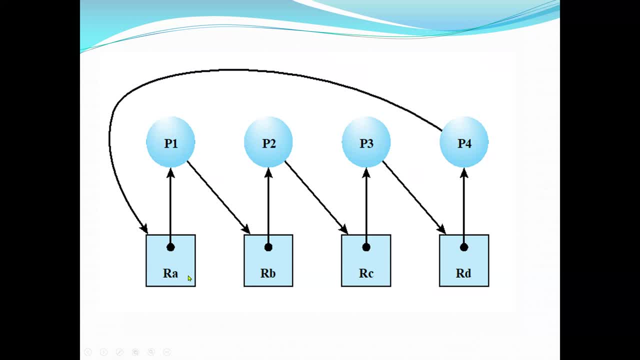 so that's the circular concept also. so here we have a resell resources are, they are reusable resources is granted to p1, rb to p2, rc to p3, rd to p4, but p1, half r a is requesting for rb, p12 b is requesting for. then it again goes all up all the way. it's a kind of a concept of a circular. 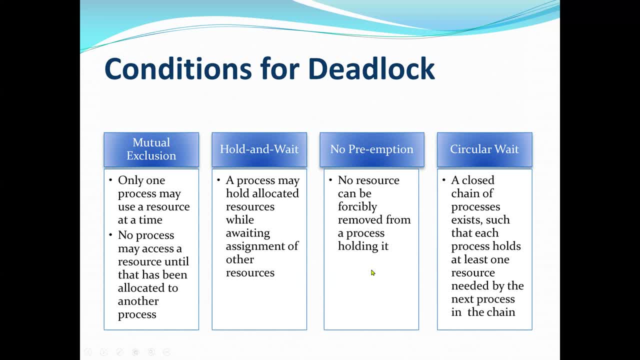 weighting. so again, that's a, as we can see, this is a circular weight concept. so the next is the condition for deadlock. so we have four conditions here, sorry, three conditions of a policy that we again need to follow. so three condition of policy must be present for deadlock to be possible. so first is the mutual excretion. so mutual excretion means again only one. 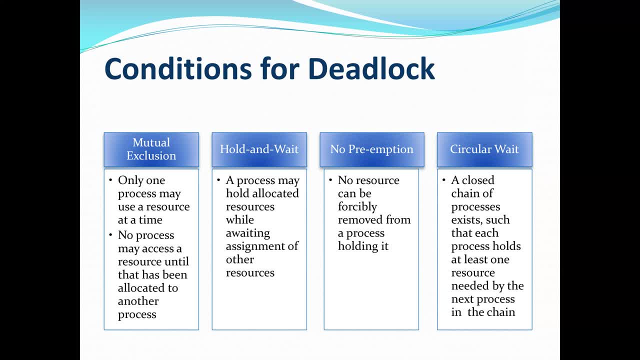 process may use a resource at a time. no process may access a resource on unit that has been allocated to another process. the next is hold and wait. so hold and wait again. process may hold allocated resources while waiting assignment of other resources. then we have the no preemption. 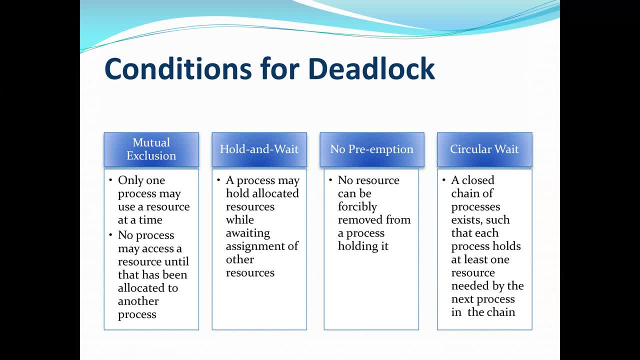 that said, no resources can be firstly, or possibly removed from a process holding it. so again, in many ways these conditions are quite desirable. example will be: the mutual excretion is needed to ensure consistency of results and the integrity of a database. similarly, preemption should not be done arbitrarily. 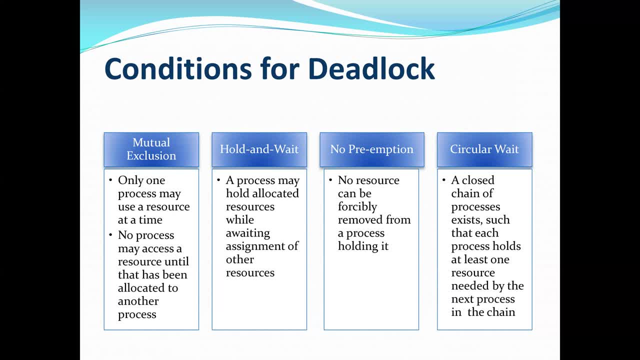 for example, when the data resources are involved, preemption must be supported by a rollback recovery mechanism which again restores the process and its resources to a suitable previous state, from which the process can eventually repeat its action. also, we have the circular weight, which is a closed chain. 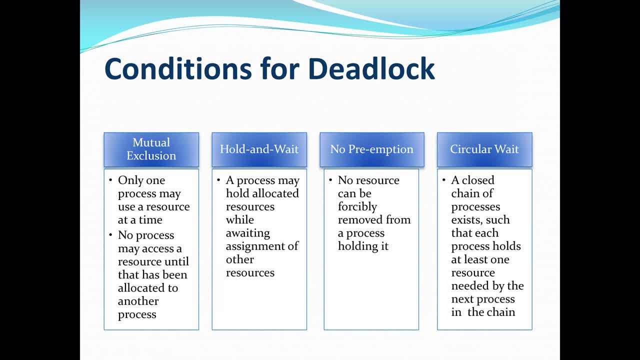 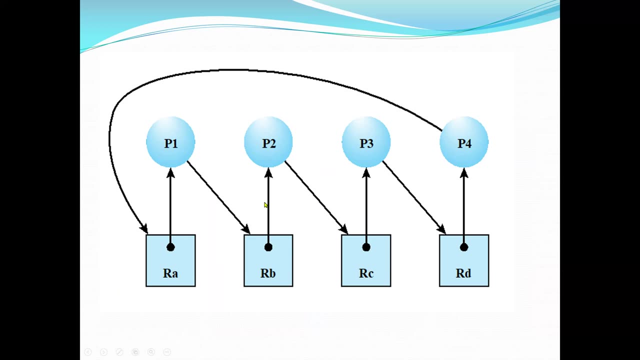 of process exists such that again, process hold at least one resources needed by the next process in the chain, as we saw in the previous slide. so this is circular: p1 half array is looking for rb, p2 of rb looking for rc, requesting for rc, and it keep going. 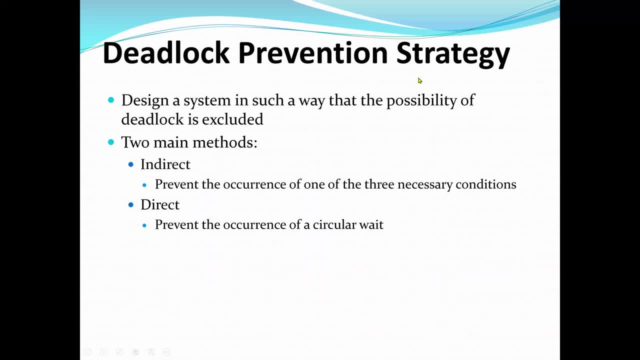 so now we need some field deadlock prevention strategy. and here we said again: design a system in such a way that the possibility of deadlock is excluded. so we have two way of doing this, two method: indirect or direct. so the strategy of a deadlock prevention is simply put to design. 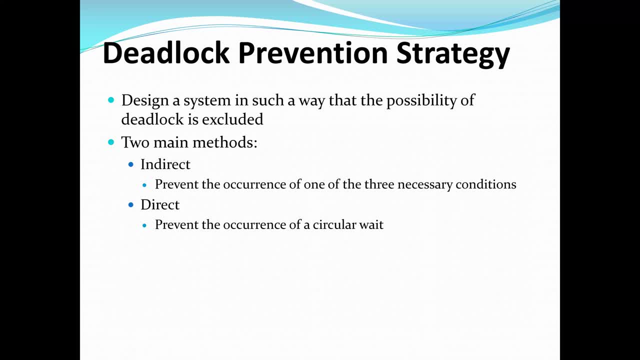 a system in such a way that again the possibility of deadlock is excluded. now we can view deadlock prevention method as falling into two cases, as indirect method of deadlock prevention is to prevent the occurrence of one of the three necessary conditions listed in our previous slides: the three conditions excluding the circular weight, then the direct. 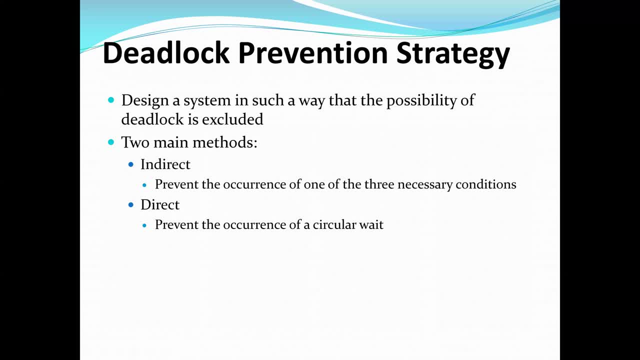 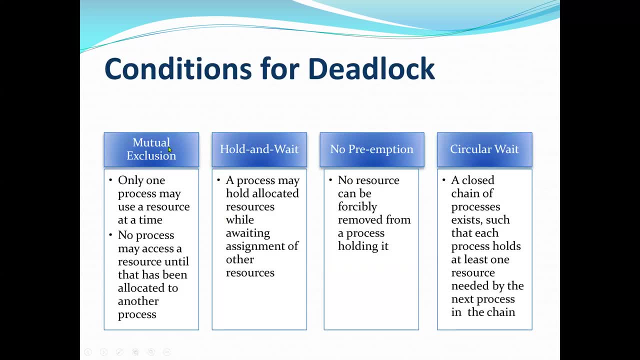 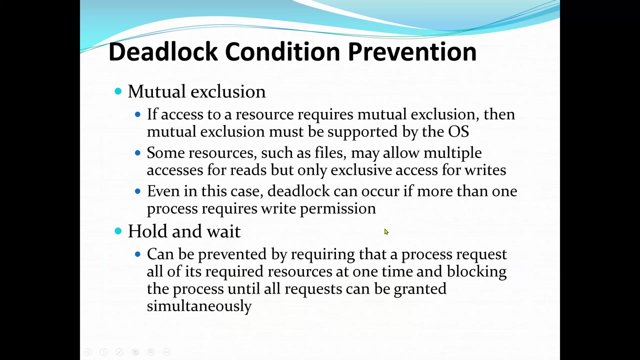 method of deadlock. prevention is to prevent the currency of a circular weight. so again we can go to the previous slide. the first, indirect, mutual excretion: hold and weight and no preemption. then direct also we should exclude, prevent the occurrence of circular weight. so a mutual excretion here. we say that in general. the first of the four listed condition: 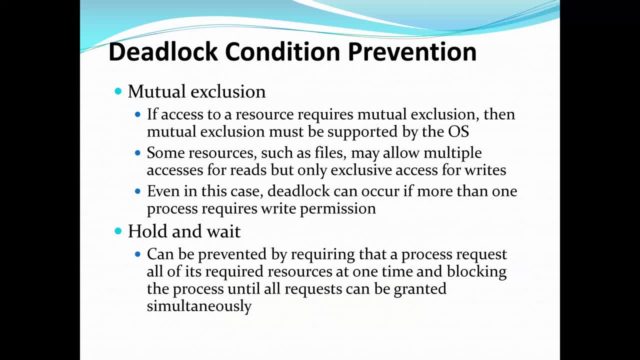 cannot be disallowed. cannot be disallowed. if access to a resource require mutual excretion, then the mutual excretion must be supported by the operating system. and also some resources, such as files, may allow multiple assets for reads, but only exclusive assets for right. even in this case, a deadlock can occur if more than one process 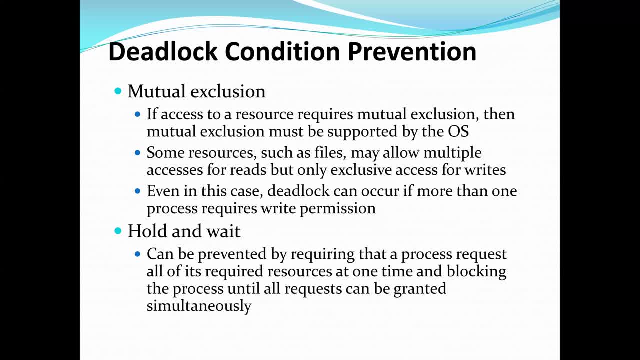 again requires right permission. so again we say: even in this case the deadlock can occur if more than one process require the right permission. also, the old and weight condition can be prevented by again requiring that the process request all of its required resources at one time only and block the process. 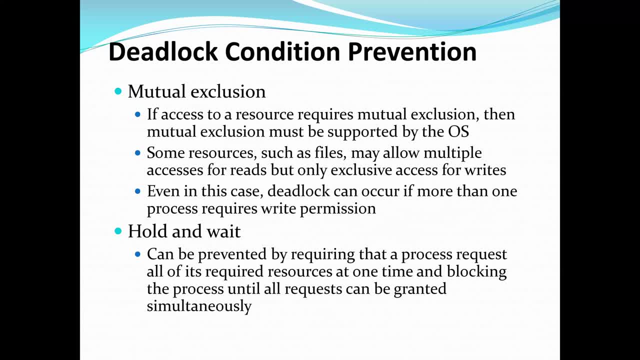 until all the requests can be granted simultaneously. Again, this approach is inefficient in two ways. First, the process may add up for a long time waiting for all of its resources requests to be filled, When actually, in fact, it could be proceeded. 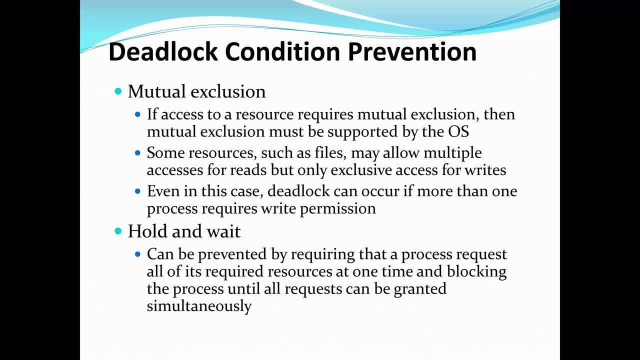 with only one sum of the resources. Second, resources allocated to a process may remain unused for considerable period, during which time they are denied to other process. So another problem is that the process may not know in advance all of the resources that it will require. 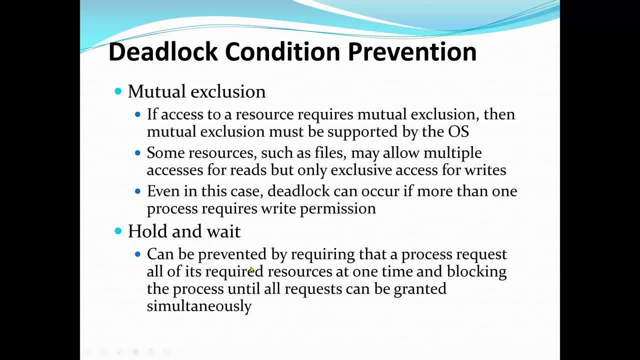 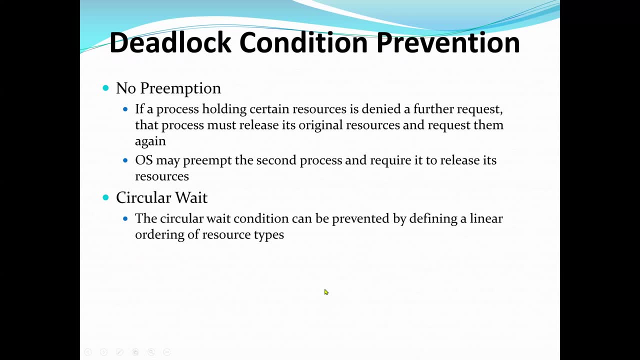 That's the concept of order weight, can be again prevented by requiring that a process requests all of its required resources at one time, then blocking the process until all the requests can be granted simultaneously. Then we also talk about the no preemption. Yeah, we'll say that if a process 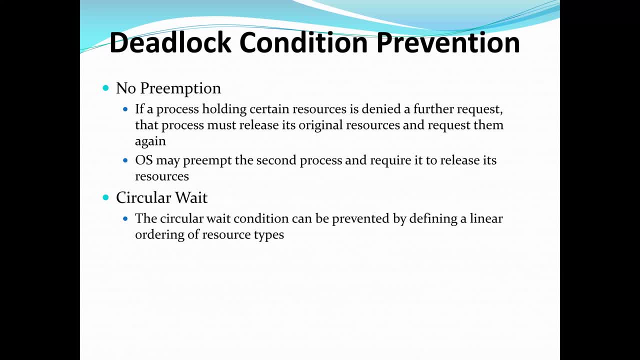 holding a certain resources is denied a federal request, that process must release its original resources and request them again. So pretty system may preempt the second process and require it to release its resources. So this approach practically only when applied to resources whose state can be easily saved and restored later. 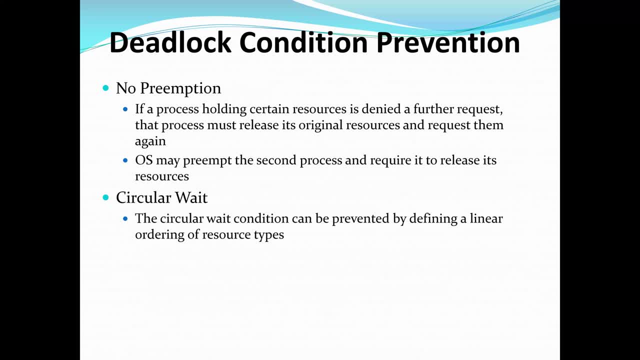 as in the case with a processor. So if a process requests a resources that is currently held by another process, the operating system may preempt the second process and require it to release its resources, And the circular weight again condition can be prevented by defining the linear ordering of resources steps. 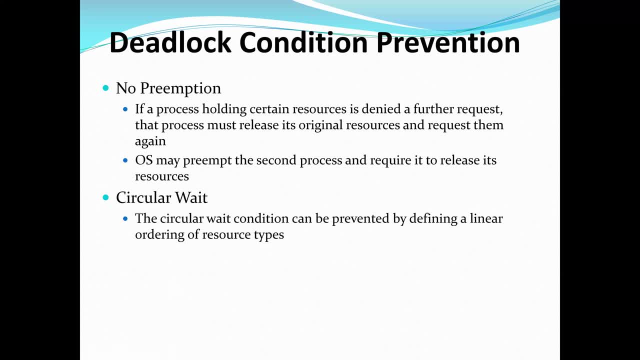 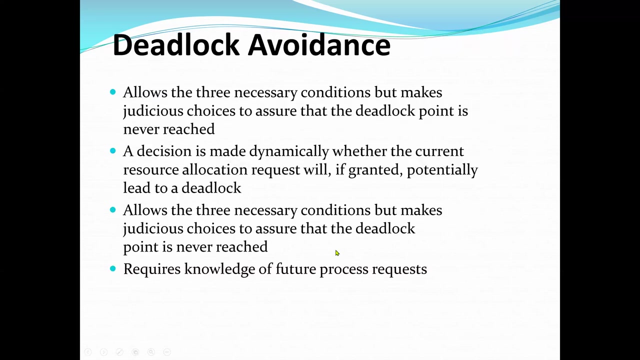 If a process has been allocated resources of type R, then it may subsequently request only those resources of types following in order. So that is, the circular weight condition can be prevent, but and defining linear order of resources steps Now. the next is the deadlock avoidance.